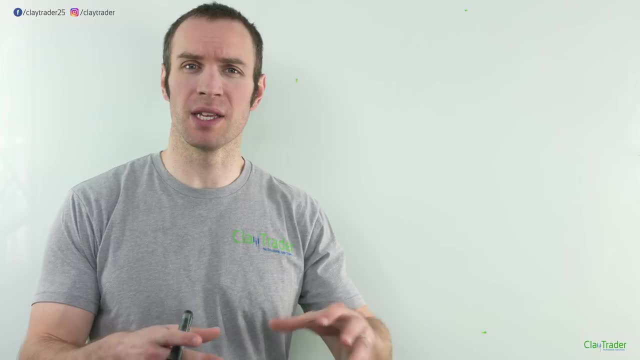 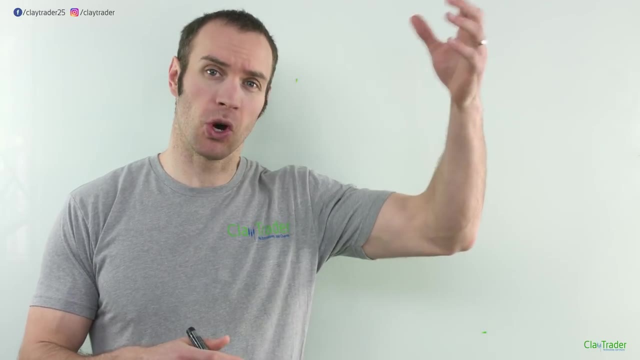 And you can go and watch that if you want. but you know that video essentially, in a nutshell, is supply and demand. When people want shares, when people want stock- and a lot of people want it- prices will go up. 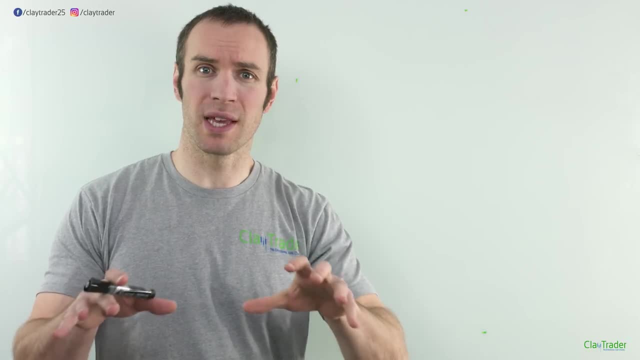 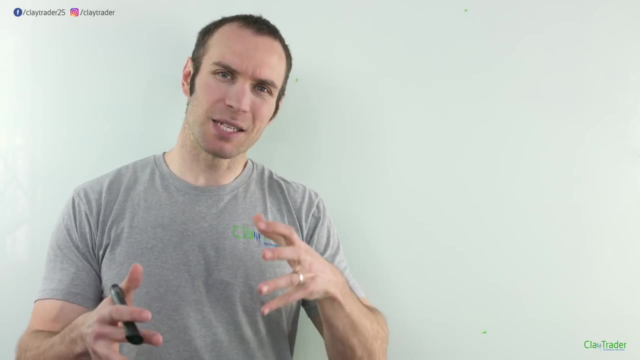 When people don't want it, when people, you know, wanna sell what they've already owned and bought, then that's where prices are gonna go down. But I got this question on a YouTube comment and it's pretty much asking, I think, another layer deeper. 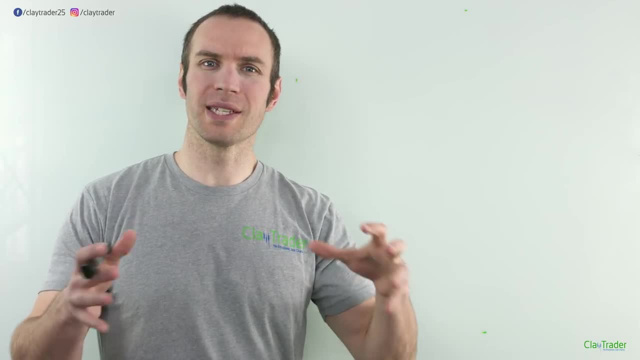 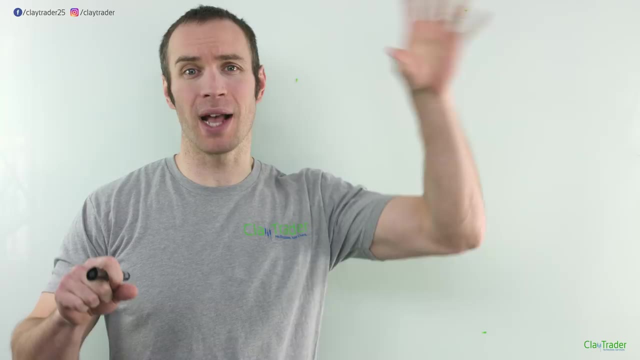 So, going down another layer in terms of you know what is actually, you know, directly affecting a stock and its pricing, yes, again, overall supply and demand. When people want something, it's gonna go up in price. When people don't want it, it's gonna go down in price. 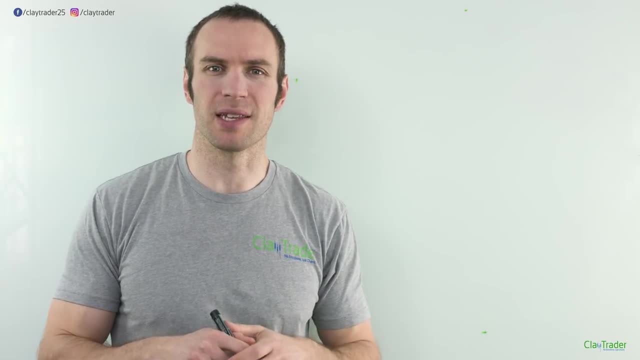 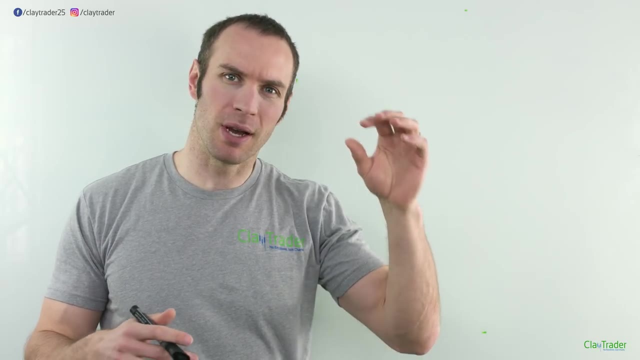 It's gonna go down in value, But what is actually directly affecting this? So let's first get to this comment and then, you know, we'll get into- hopefully, me being able to describe this at a little bit more of a narrower level. 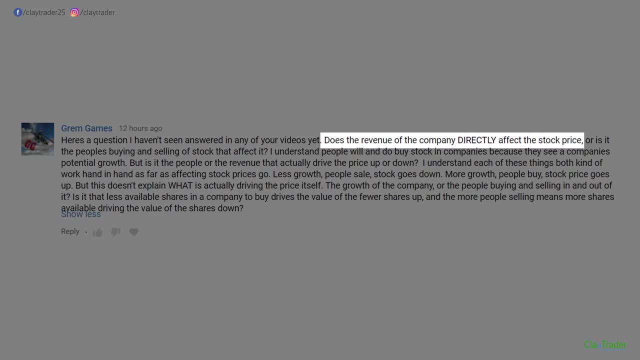 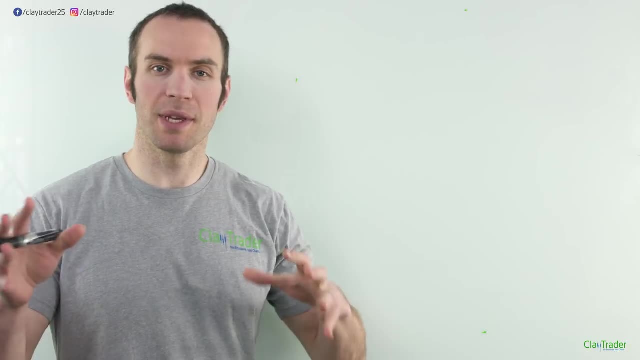 Now this person says a lot more, but I wanna just kinda focus on one comment in particular. They say: does the revenue of the company directly affect the stock price? This whole concept is there's a lot of gray area, because now that brings up the question. 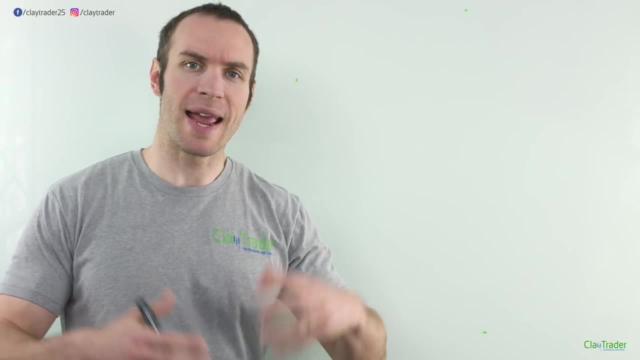 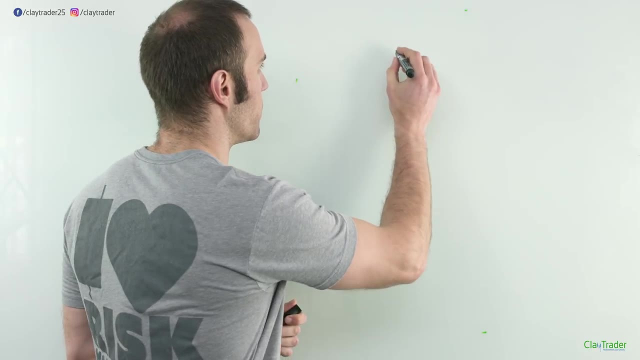 well, how are you defining directly? What do you mean by directly affecting? And at its core, I like the way this was phrased because it brings up a dynamic of the market's revenue, And revenue is just pretty much how much money. 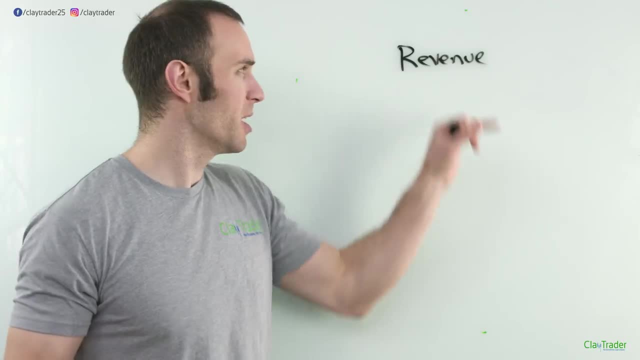 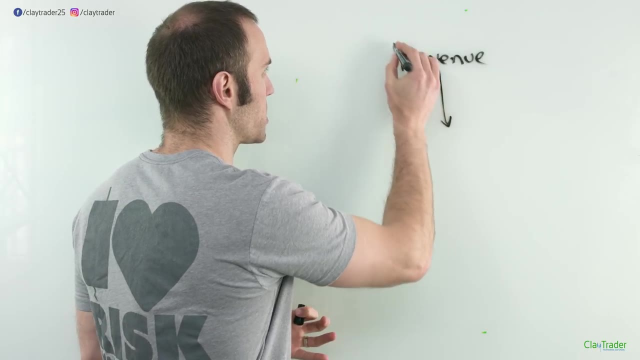 a company is generating, Not the profit- but this is not an accounting class- but just how much money is a company generating from its sales. And on this- this being a piece of paper, you know you have all sorts of documents that companies have associated with them. 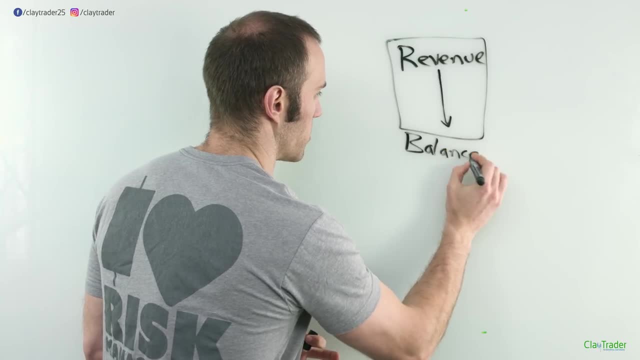 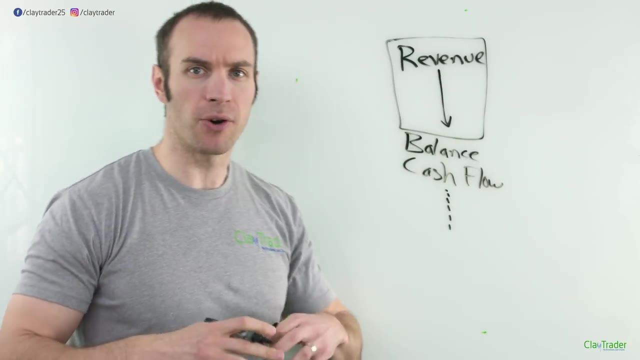 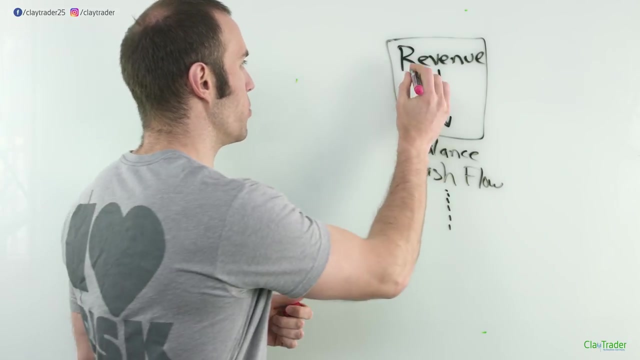 You know, you have balance sheets, you have cash flow statements and you have lots of other different things that tell you about a company, tell you how a company is doing, And the person's question is all right. so in this case, you know revenue. 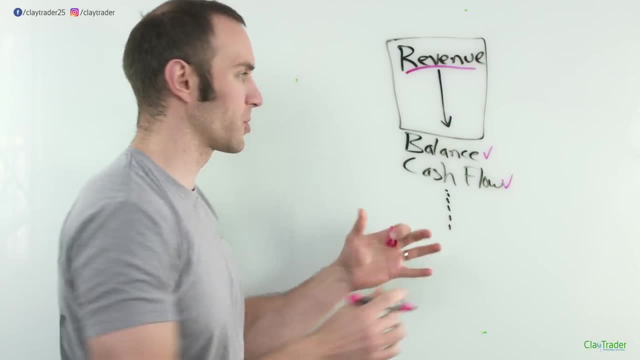 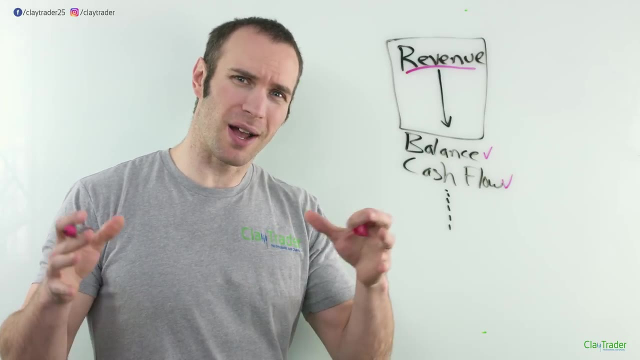 but you could definitely fill in the blank with any of these other things. Is that directly affecting the price? No, It is affecting the price. It is, but it isn't. And this is where I don't quite understand what this person is saying by directly. 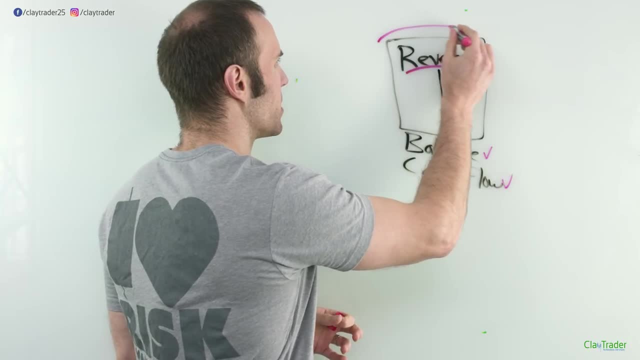 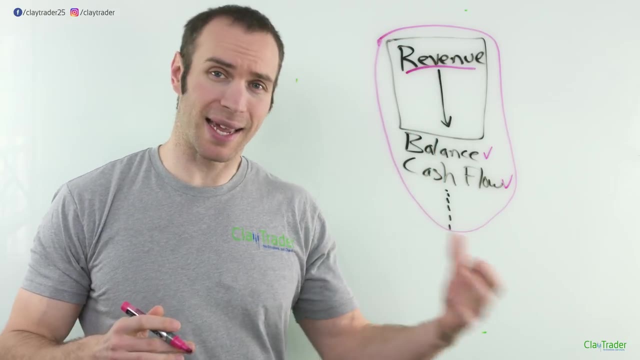 but I do know what they're understanding. But my point here is the thing that is ultimately directing the price and affecting the price is not- and I kinda lied, I guess, in the video I referred to down below, because I was saying it's all about wanting. 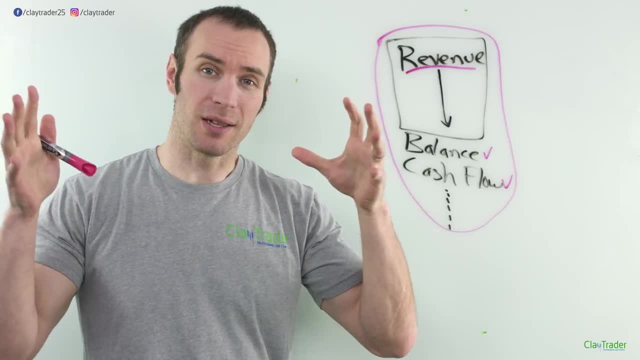 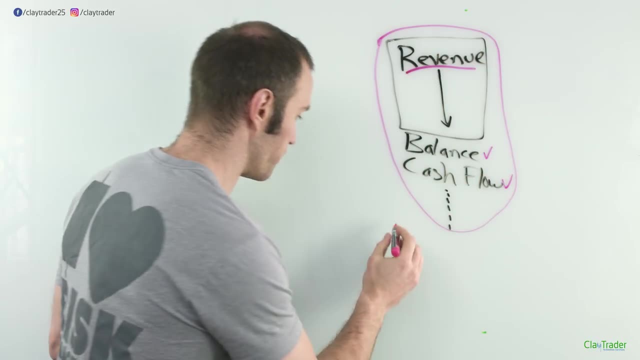 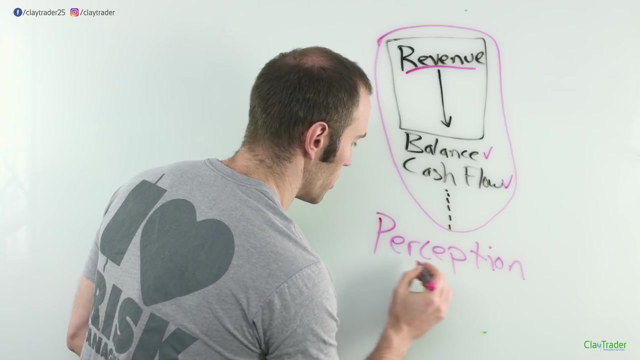 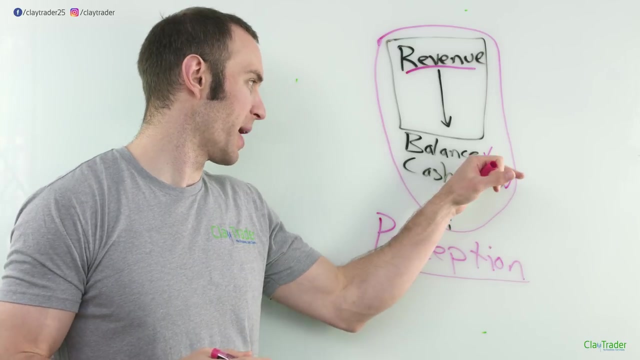 people not wanting supply and demand. There's actually another layer that encapsulates both supply and demand, you know, and then revenue, and that is just called one word, Perception, Meaning. what do people think about the revenue? What do people think about balance, cash flow, all of that? 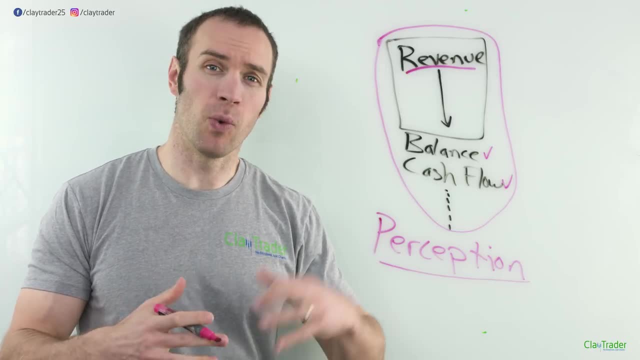 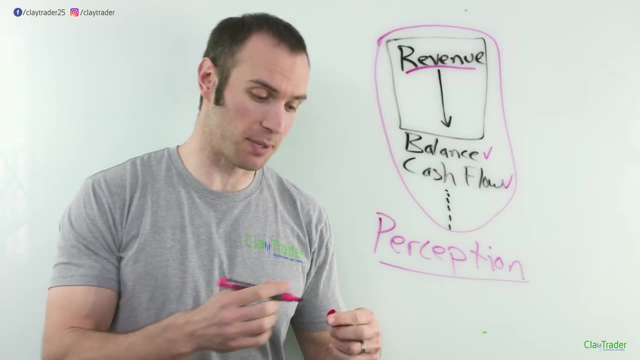 What do people think, what do people perceive about what they think may happen in the future as far as growth or maybe not growth, That is what's actually affecting the stock price, because with somebody's perceiving, or with somebody's perception, what they're perceiving, 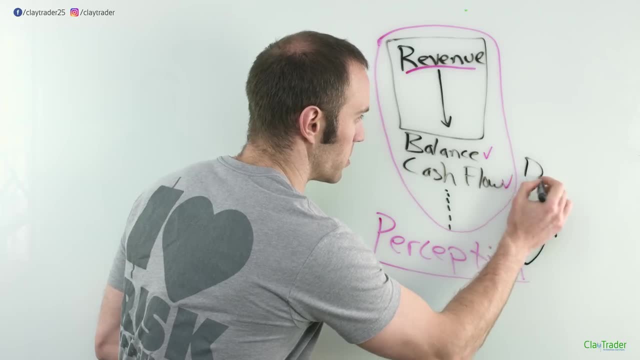 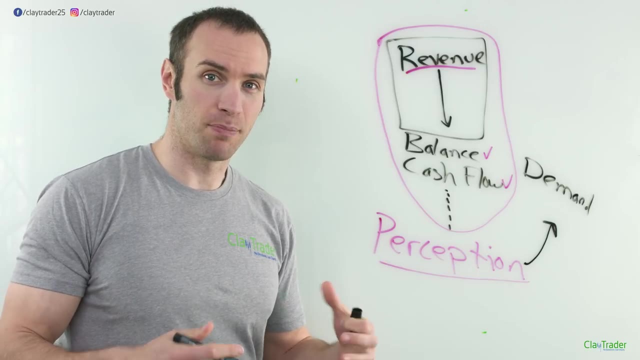 what's that gonna do? Well, that's gonna go, and then that's where the demand may come from. Or if they're not, you know, their perception is. what they're perceiving implies it that's where maybe the supply is coming from. 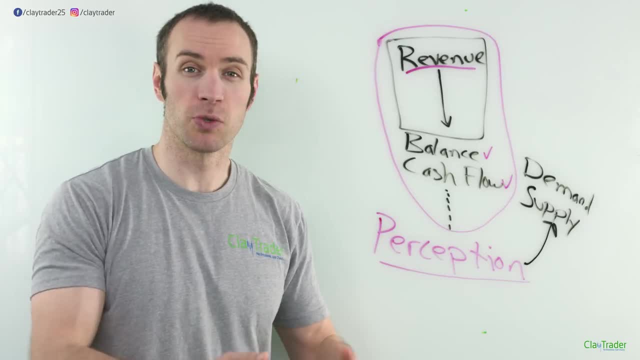 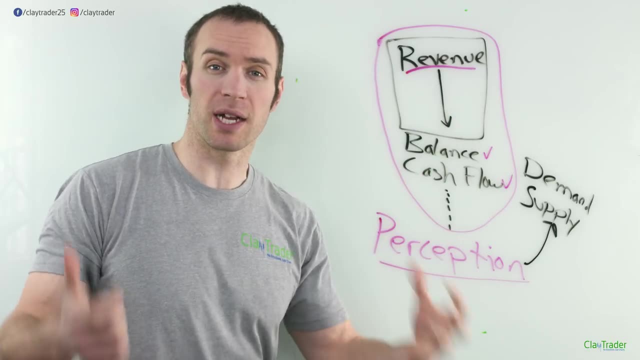 Or in other words, people wanting to sell, And that's where prices would go down. So it's all about perception. Does revenue directly affect the stock price? Does it directly affect it? I would say no, it doesn't directly affect it. 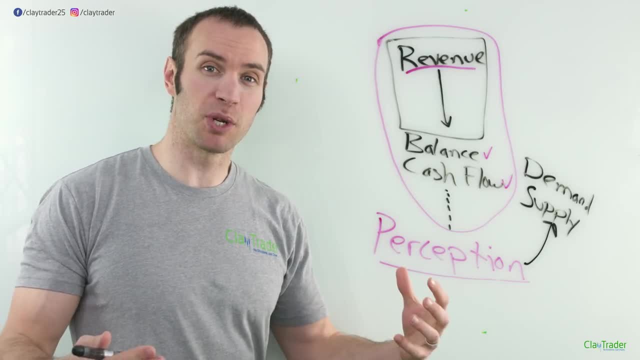 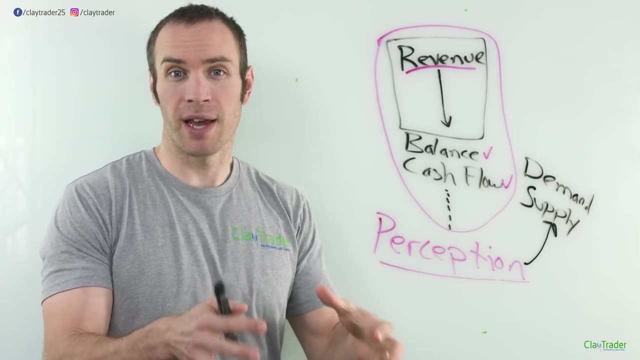 What directly affects things is the perception, because perception is then going to cause people to go and make choices that are either creating demand or supply for that stock And to pay based on that. that is where the price- and what is going to affect the price- comes from. 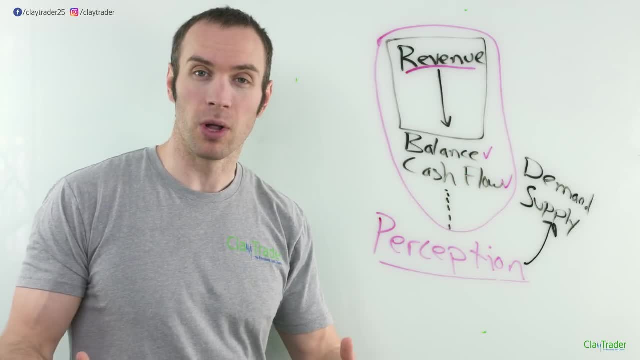 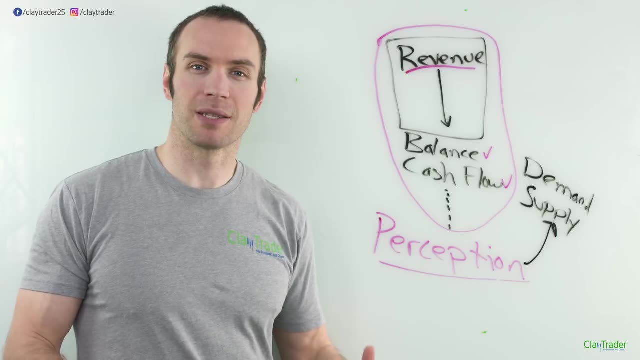 Revenue, all this sort of stuff. it without doubt plays a role, But is it the direct effect? I would argue no, and we could probably get into a big semantics And philosophical argument about this, And I'm aware of that. But I mean as far as just trying to keep, 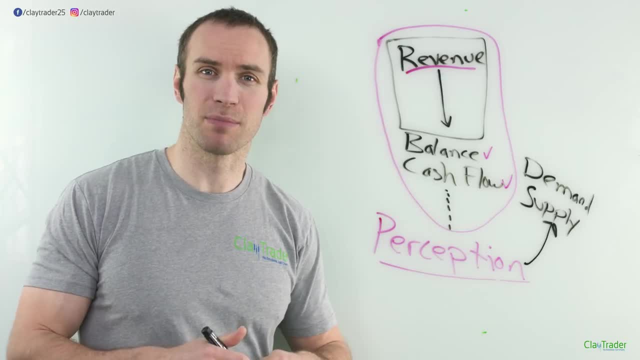 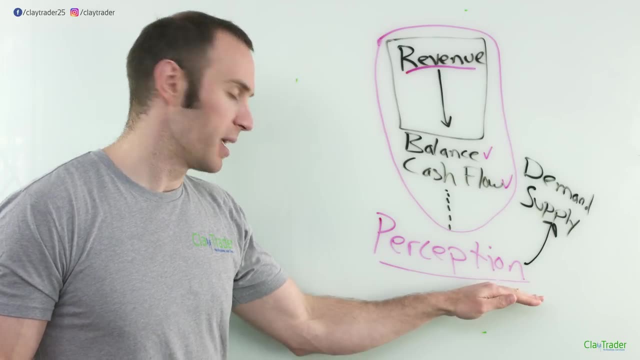 remember this is in the Trading 101 section of the site, so this is not like some sort of. I'm not trying to make this overly complicated, But just answer these sorts of questions in terms of directly affecting the price. At the end of the day, it's all about perception. 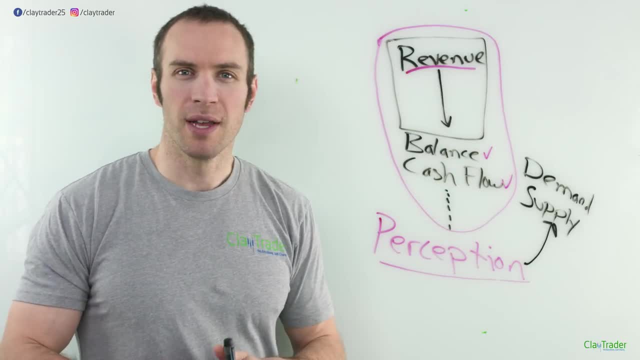 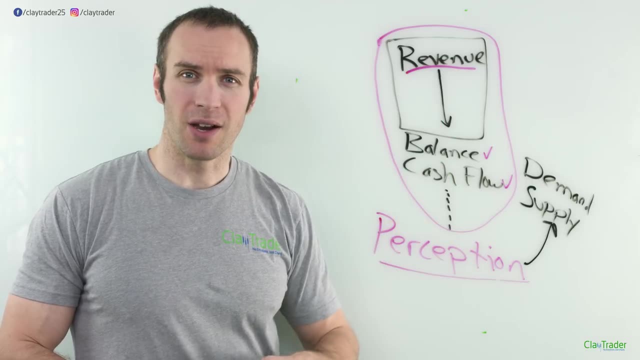 How people perceive revenue. Quick little example, and you know you can do this if you want, but what I like to do is you know a company will release their earnings And I will go down and read through things and say, oh well, geez, I am perceiving that, as you know, 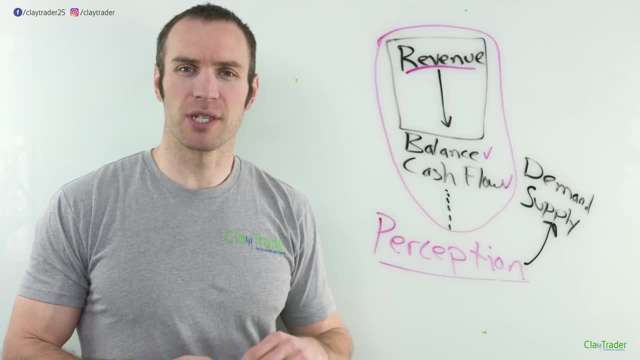 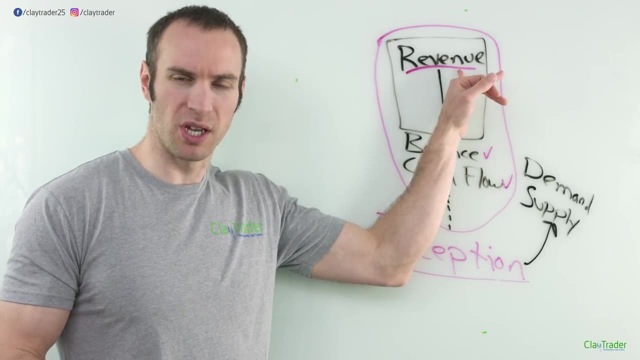 I am perceiving that as revenue. That sounds good, that sounds good, And then you watch the stock that day and the price goes totally down. Well, which is the case. Well, revenue was good, You know. the cash flow was good. 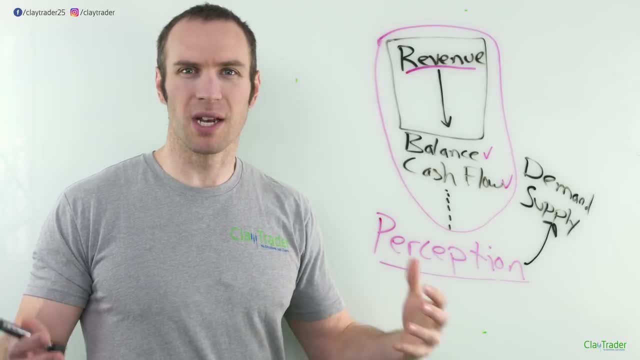 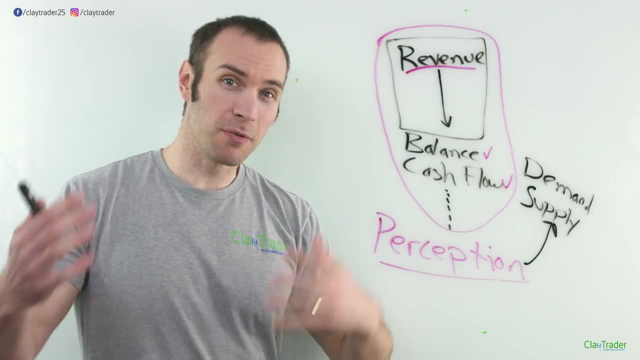 The balance statement was good, But then the price goes and does something totally else. Well, that is because the perception of what I'm seeing, my perception, is different, So everybody's perception is gonna be different, and that's what makes a stock market. 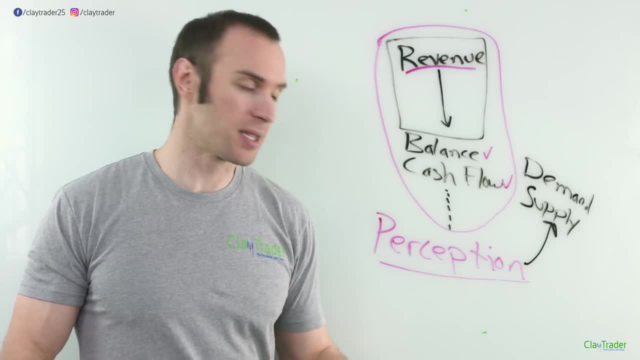 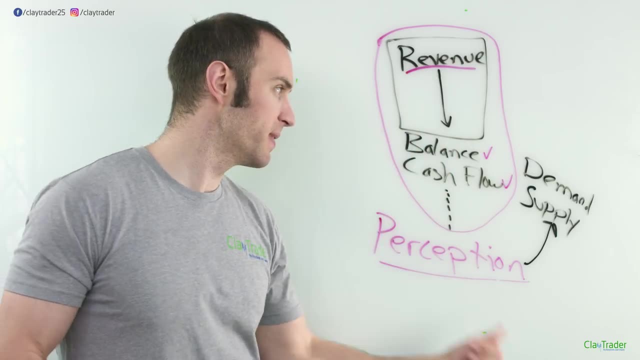 such a fascinating thing. It makes it the ultimate game upon games, because it's who's best at perceiving what is actually going on. Revenue is just a number, but how that number is perceived is what's gonna dictate demand, what's gonna dictate supply. 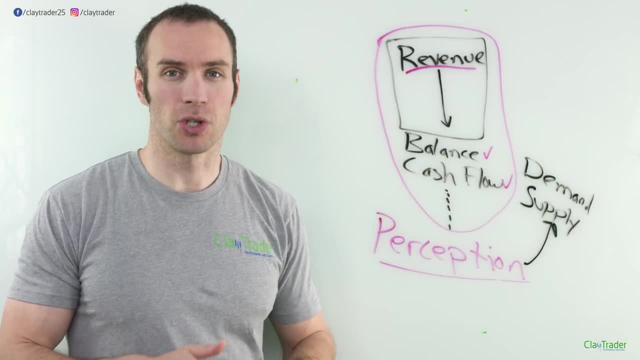 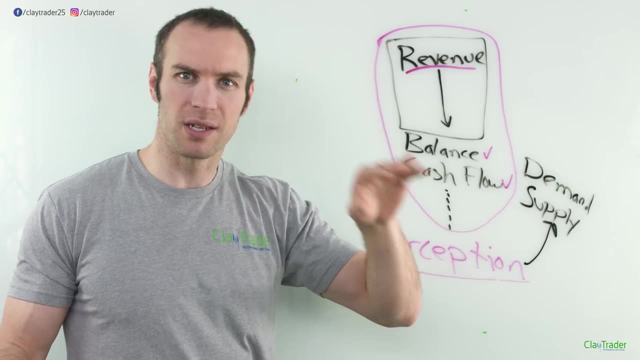 and that's what's gonna ultimately dictate. you know how a price unfolds, So I don't know if I answered the question. I think I did, but it's a hard question. But revenue, all this stuff directly, no. 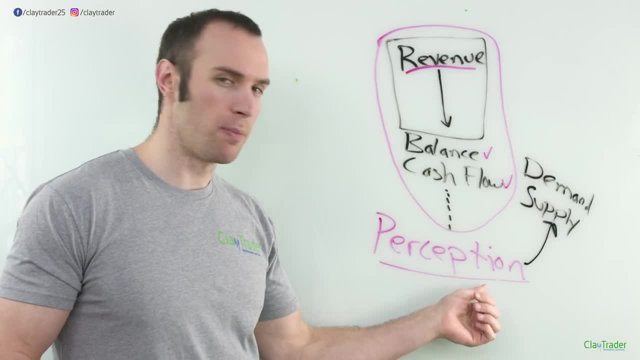 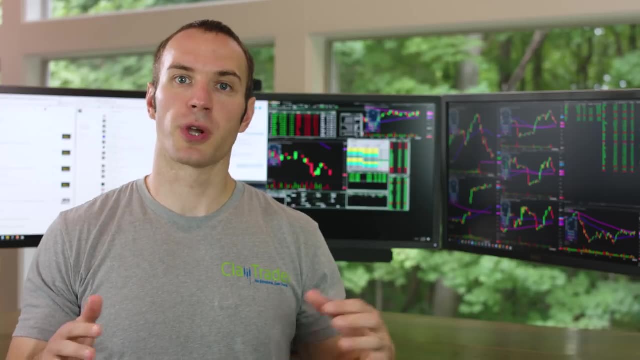 it does not directly. it plays a role but at the end of the day, it's all about perception and how people are perceiving revenue and the other dynamics within the market. If you are out there trading alone currently and maybe are in the market looking for a community to join, 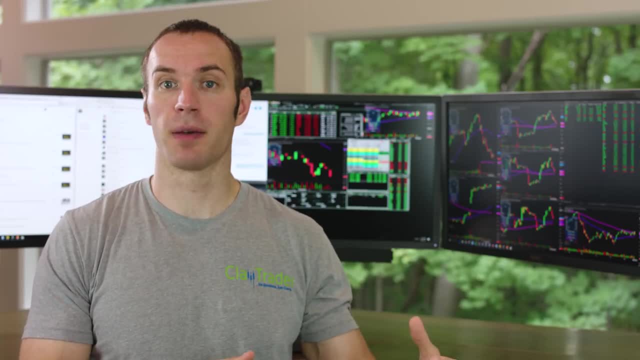 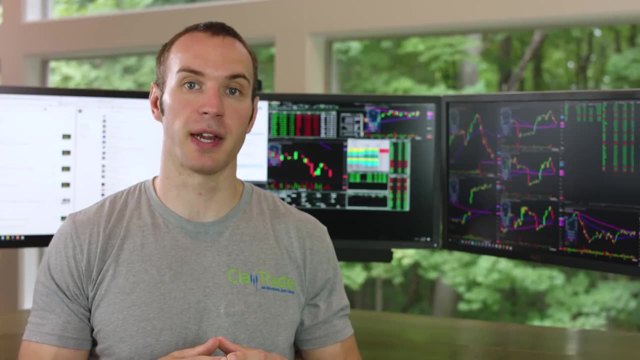 to assist you in your trading, or to just help you, you know, give you another set of eyeballs. then I do have a private trading community where you can trade alongside me and other experienced traders. So what you see popping up on the screen right now. 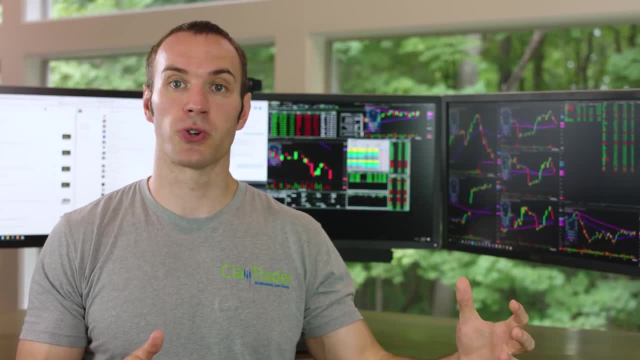 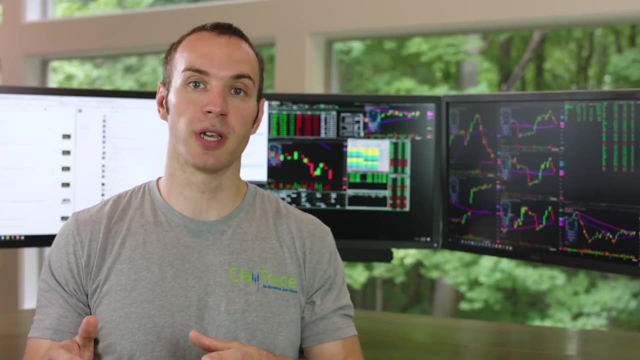 is both an information link, so if you click on the inner circle, one that is going to take you to the page where I explain all the details of what exactly come with the community, both the chatroom and the newsletter, and then the other image that has popped up. 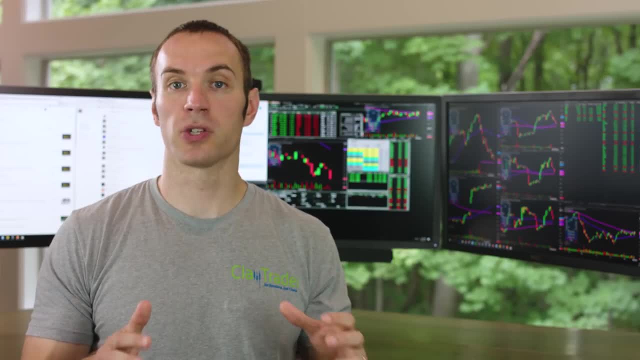 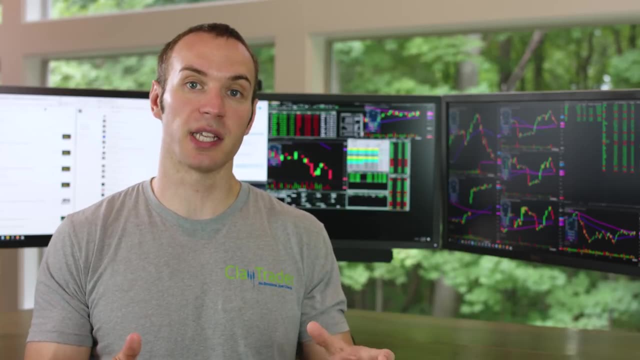 is a behind-the-scenes tour where you can see exactly what is going to, you know be contained within the community. I take you through, like I said, a behind-the-scenes tour of everything and that way you'll know precisely what you are getting you know when you join. 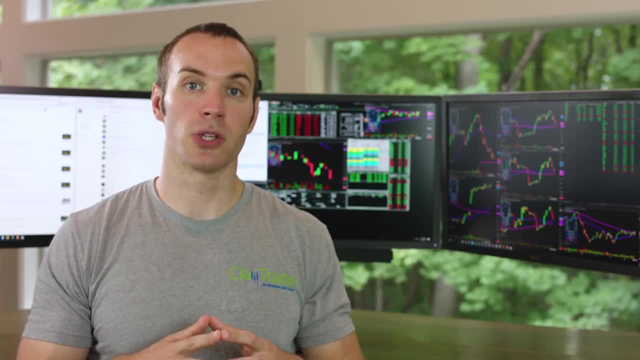 So definitely check that stuff out if you are interested and thinking about, you know, wanting to join a community and let me know if you have any questions.